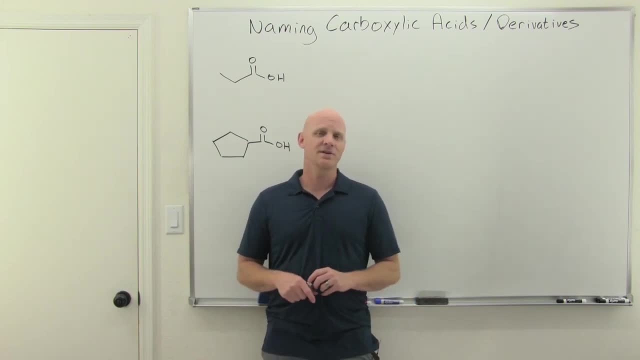 Again, 99% of you are never going to see them. You're never going to see these function groups named as anything other than the highest priority functional group. Now, this lesson is part of my organic chemistry playlist. I'm releasing these lessons weekly throughout the school year, So if you want to be notified every time I post a new, 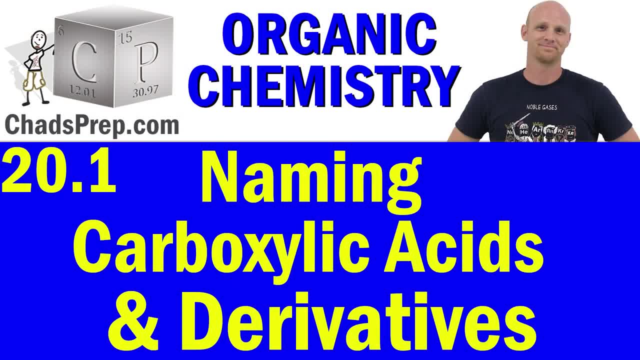 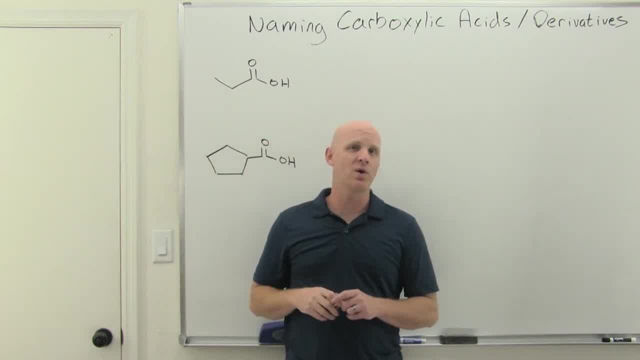 one. subscribe to the channel. click the bell notification. Okay, we are going to name these in descending order of priority. So these are the head honchos on your priority list of organic functional groups and their nomenclature, And so the highest one, that's going to be carboxylic. 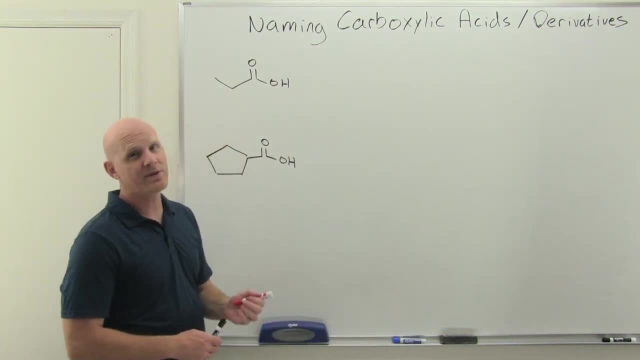 acids, And that's what we're going to be naming. So we're going to be naming these in descending order of priority And that's what we're going to start with first. And when you name a carboxylic acid- so, as it was with all these derivatives- we'll find out. they are always anchored to the 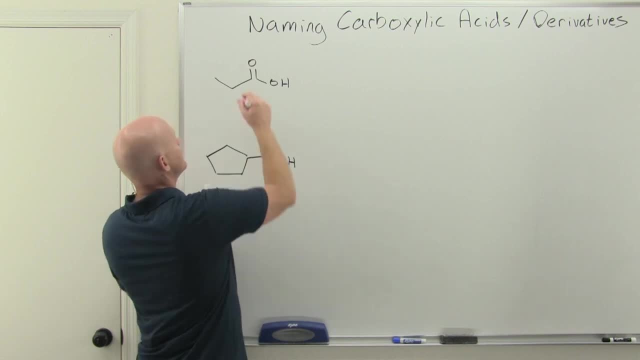 end of the chain And so, as a result, when you name them as such, so the carboxyl carbon here is going to be carbon number one And because it's carbon number one, that is, and it has to be a carbon number one, that's never going to be included as part of the name here. So in this case, 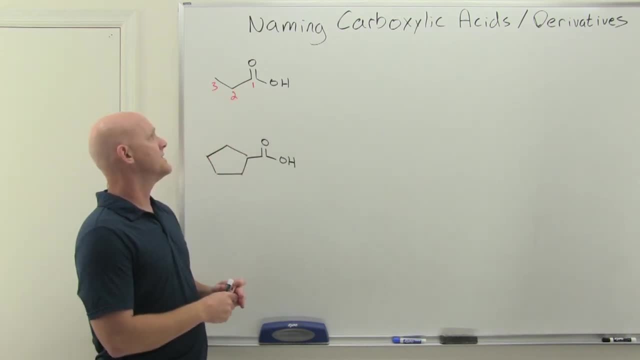 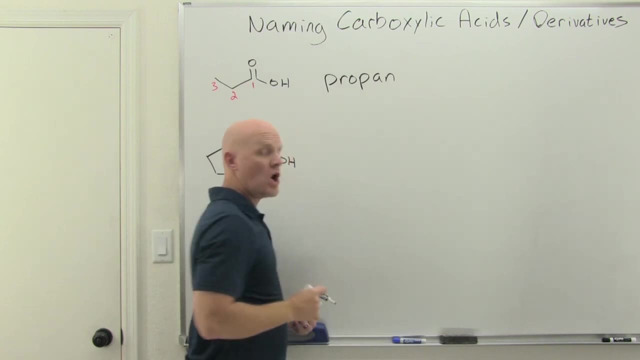 a three carbon chain is propane, And in this case the suffix is oic acid. So we're going to start off with propane And because oic acid begins with a vowel sound, we'll drop off the E and we'll throw on that. 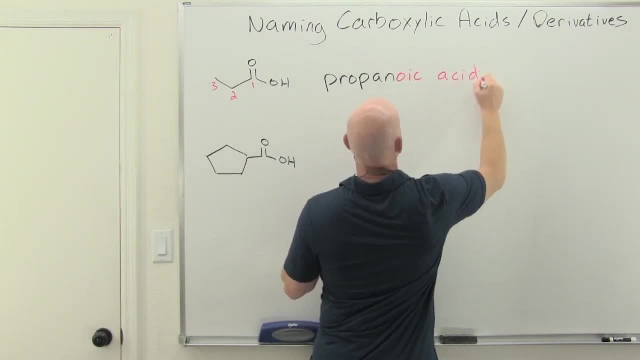 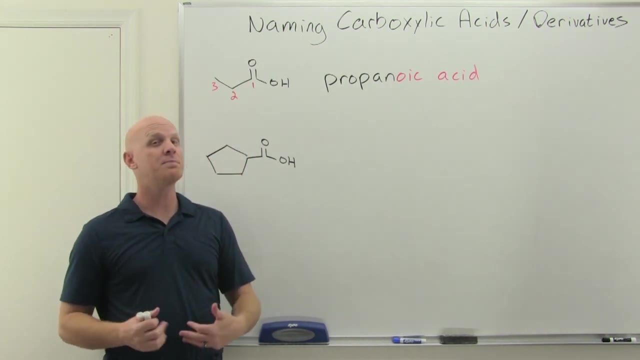 suffix oic acid, And this is propanoic acid. So in just a word of the wise, for three carbons. sometimes you'll see it written with a common name: propionic acid. might be worth knowing. Same thing with two carbons: ethanoic acid, more commonly called acetic acid, And then four carbons. 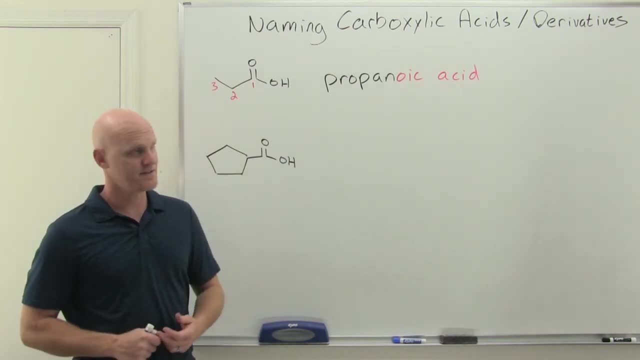 butanoic acid, also commonly called butyric acid. So just in case you see any of those common names. Now, if you've got a carboxylic acid on a ring, special case, we saw something similar with aldehydes. So if this was just an H over here and it was an aldehyde, this would be cyclopentane. 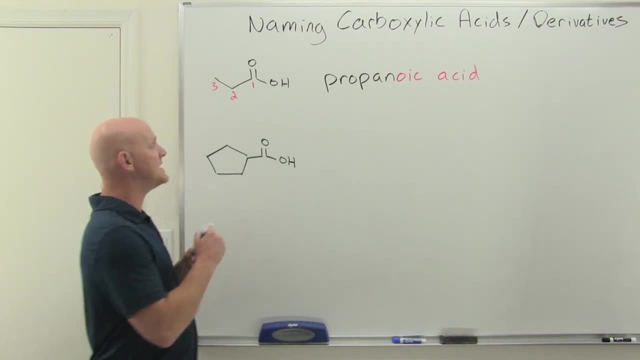 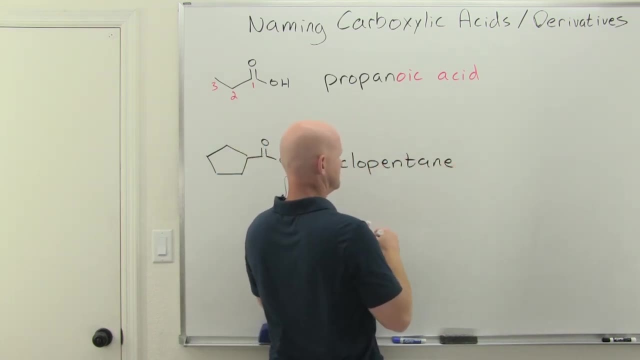 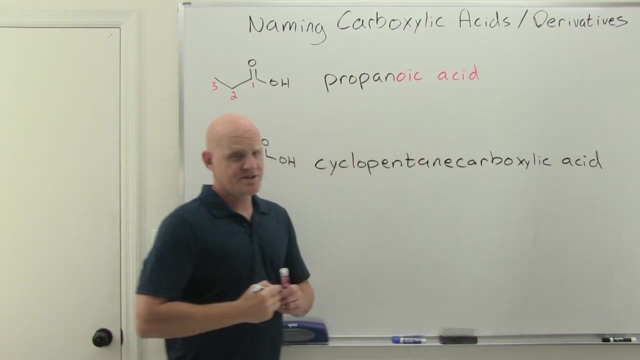 carbaldehyde. Well, in this case it's a carboxylic acid, So it's cyclopentane carboxylic acid. Cool, Just a special case if your carboxylic acid is directly attached to your ring. So we saw something similar with aldehydes. So if this was just an H over here. 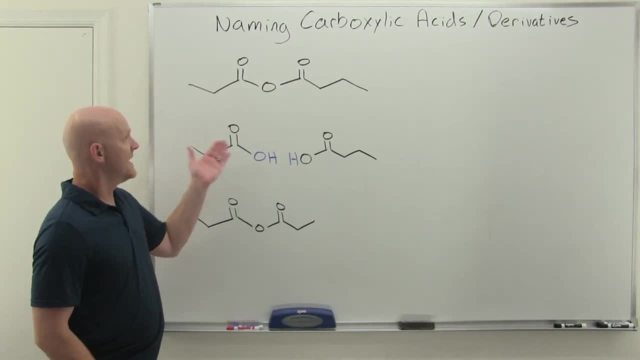 a ring. So now we'll move on to acid anhydrides. here, If you hear the word anhydride, that usually means like without water or having water removed or something along those lines, And we can see why here. So if you take a couple of carboxylic acids and put them together, you can remove the 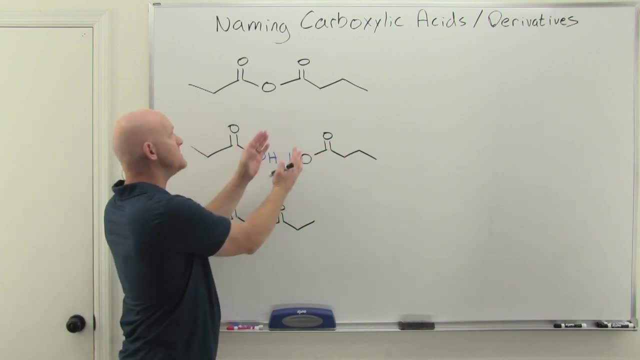 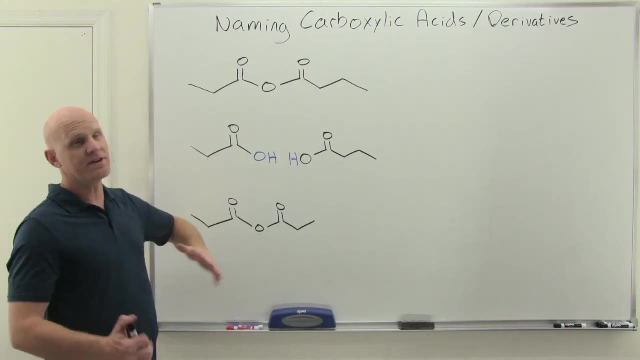 H on one and the OH on the other to form water, And then when you put them together you get this acid anhydride. Now it's not necessarily how they're formed, although they sometimes could be, but not usually- But it is kind of how they're named. So this acid anhydride, if we go to name 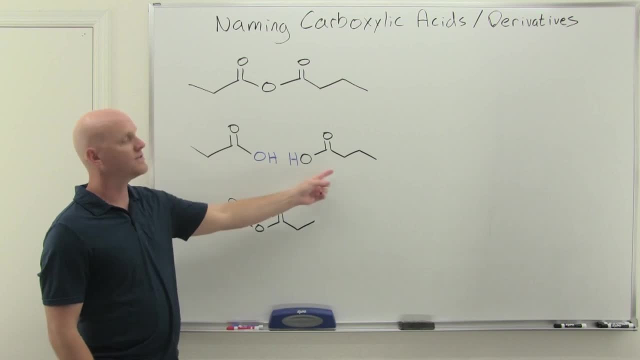 it. you got three words. You're going to name it based on the carboxylic acids it is composed of, named in alphabetical order. So this is butanoic acid, This is propanoic acid, So we'll say: 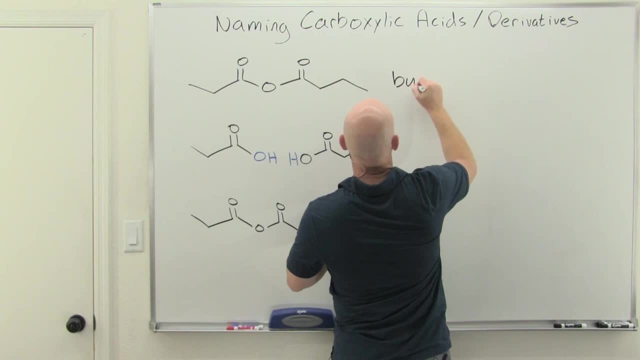 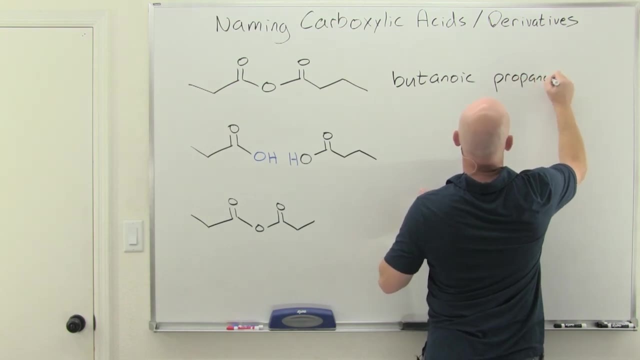 butanoic first, And so this is going to be butanoic and then propanoic, second word, And then third word's- just anhydride, Cool. So butanoic, propanoic and butanoic. 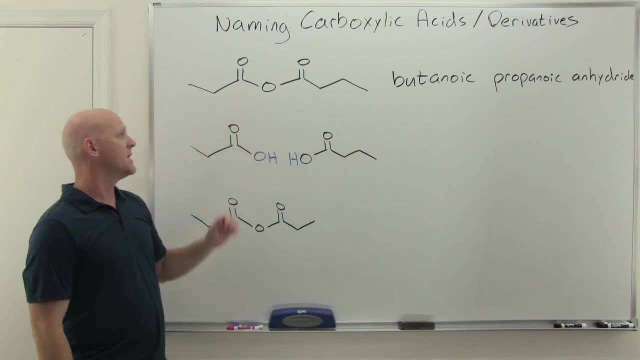 Anhydride. Now, this is what we call an asymmetric anhydride, where the two sides of the anhydride are made from two different carboxylic acids. So that's not necessarily going to be the case, In fact. 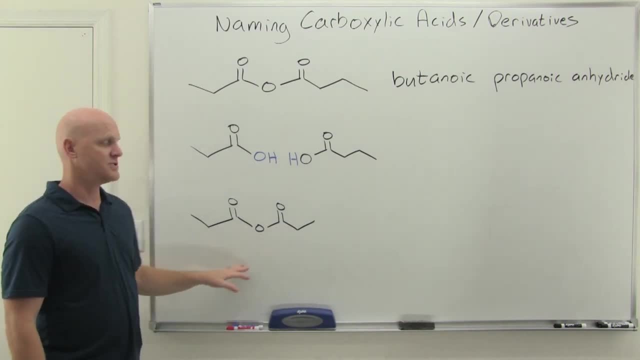 it's not usually the case. You're often going to have symmetric anhydrides And for a symmetrical anhydride like this one right here. so if you kind of follow the same thing here, well, both sides here come from propanoic acid And you'd say propanoic, propanoic anhydride. Well, to kind of 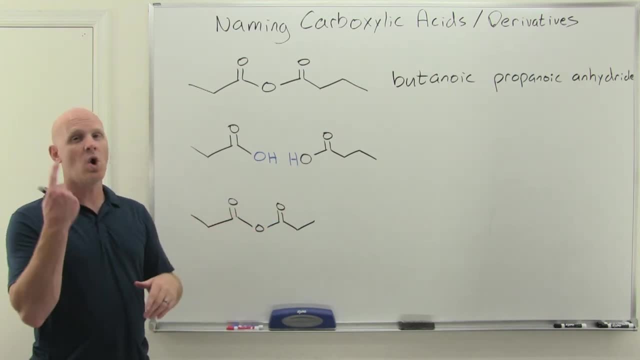 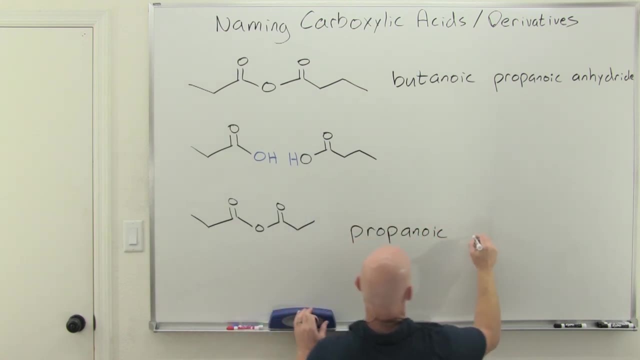 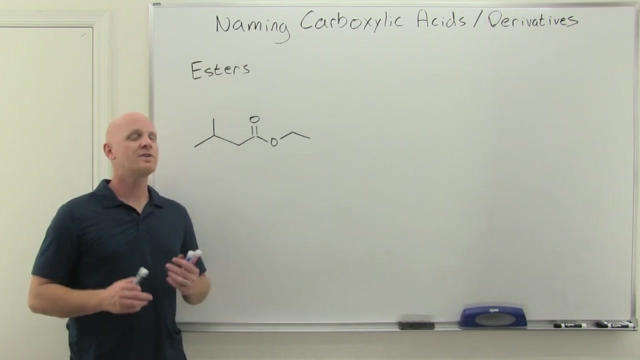 prevent such redundancy. for symmetric ones, you only use the name of the carboxylic acid once, And so this is just simply propanoic anhydride. Cool, So we've got esters next in the priority ranking. So carboxylic acids, then anhydrides. 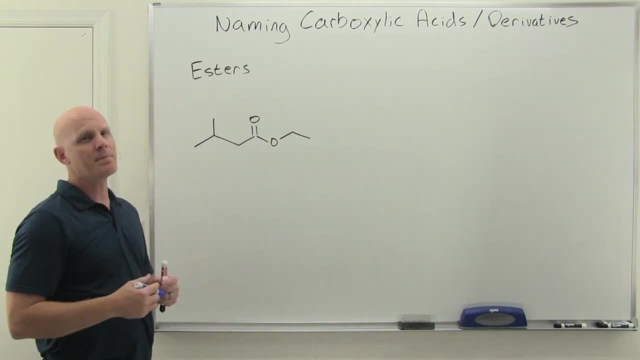 and now esters are next And esters are going to be kind of broken up in two parts here, And you've got your ester functional group here and there's the carboxyl side, which is the carbon chain containing the carbon double bonded to oxygen. 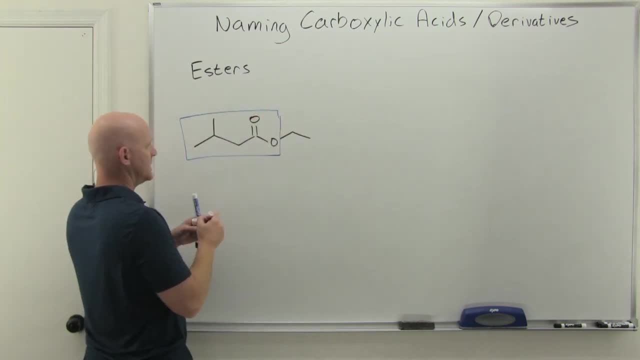 includes this oxygen. we'll kind of break it up right there, if you will so, and then this guy right here. cool, so it turns out there's two words for the ester, and the first word is just whatever. uh, you know, alkyl group is on the other side of that oxygen, right there, and so in this case that's. 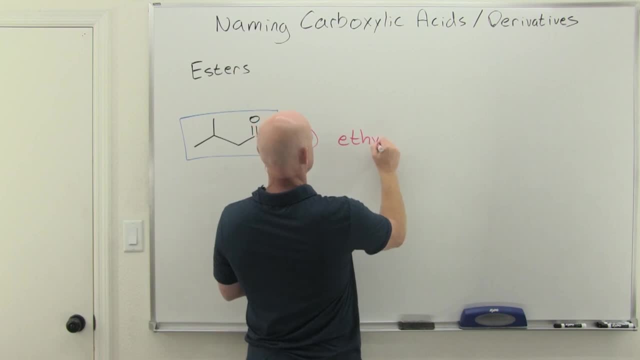 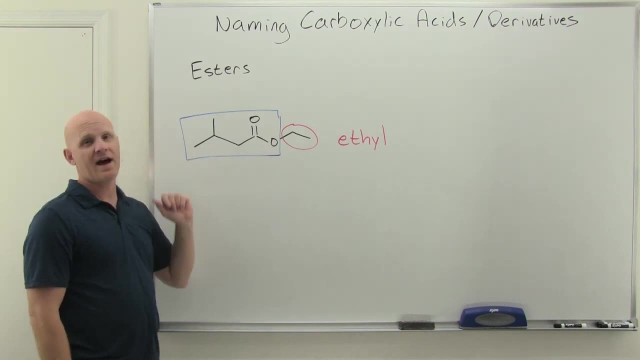 just going to be an ethyl group, and that's the first word. so we've got ethyl. so, and then this guy right here, the rest of it is actually named as the conjugate base of this carboxylic acid, and so in this case we've got a one, two, three, four carbon carboxylic acid, that's butanoic acid. 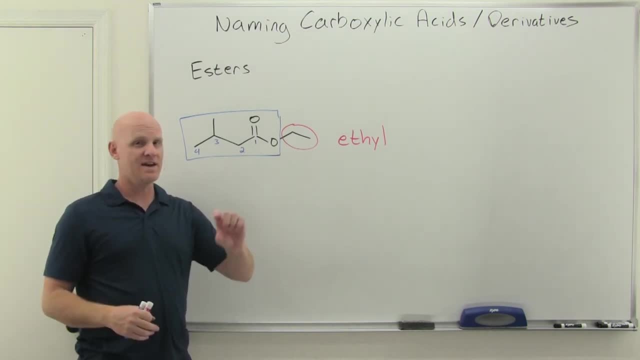 but the conjugate base is going to end with an ate, so the ick becomes eight, kind of like we did with nitric acid and the nitrate ion. it's conjugate base, same kind of thing. so it's if. if the four carbon carboxylic acid is butanoic acid, well then this conjugate base is the butanoate ion. 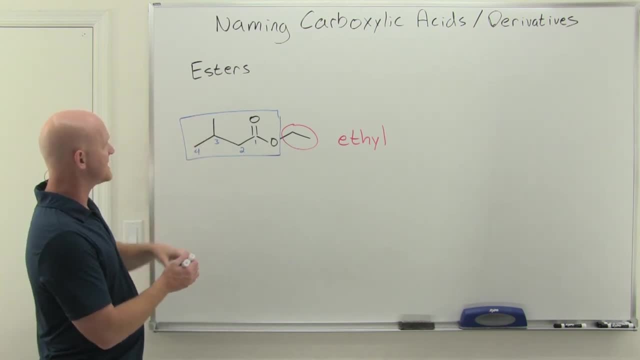 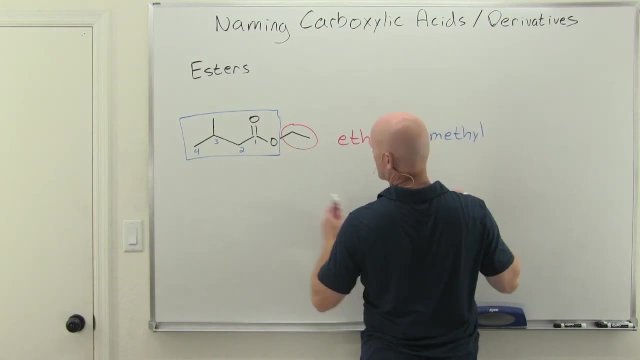 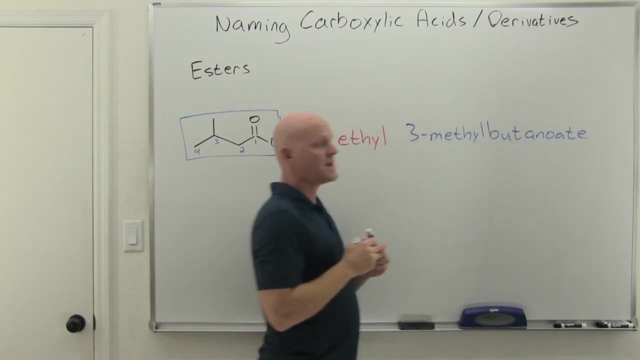 and obviously i know we have a methyl group here, we've got to throw in there as well, and so in this case this whole thing is ethyl three methyl. so right there. and then the butanoate: cool, and there's your name as an ester here. so two words again: ethyl three methyl butanoate, and 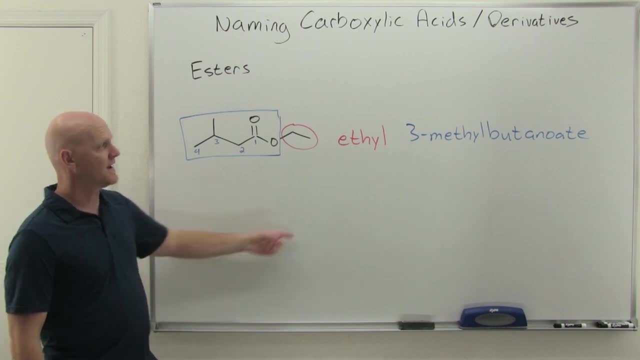 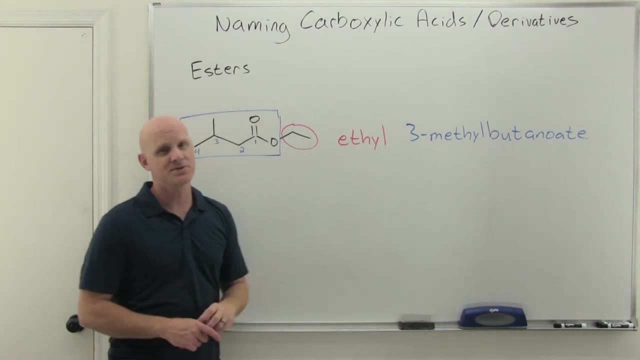 i want to make sure i put one that had an extra substituent over here so you could see the difference in why this substituent gets its own separate word. but any substituents on the parent chain itself are going to be named as part of that parent chain too. 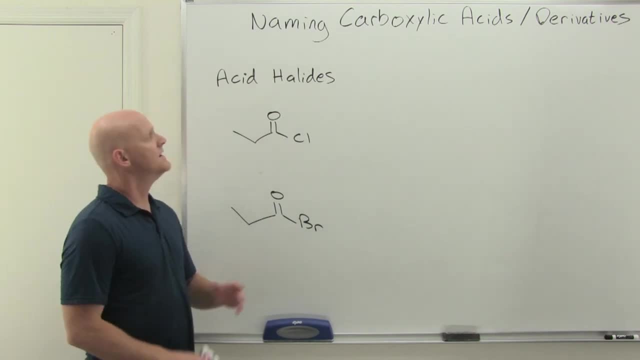 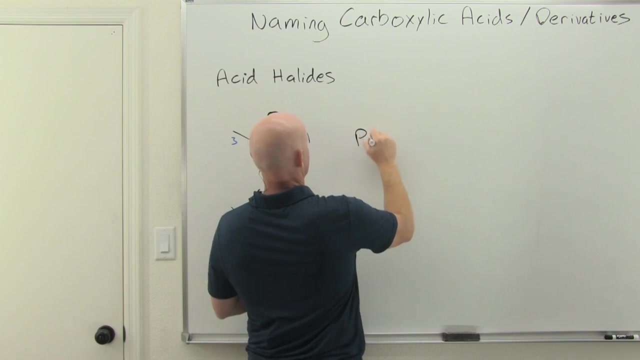 and we can also imagine that there are acyl halides in Что n. the left side and in the middle of the spiritual ethyl halide are the acyled in the right of the iron andBar II released at Wa Wanted. but they follow the same 함께 store a sphagnum. it's a natural. 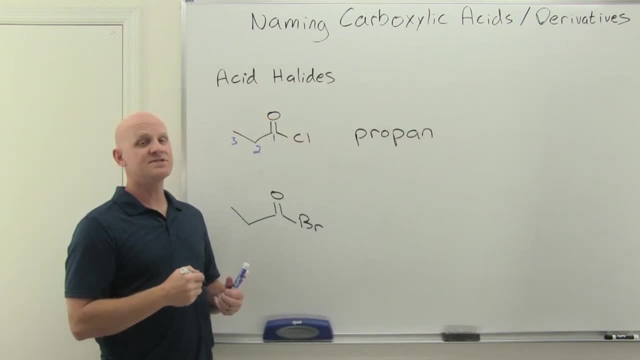 and it's the natural I'm gonna weaker, going to work the same way. in principle, number the longest chain. so one, two, three and that's propane. so so I thought it was important to translate this in different ways to make sure that we're getting the code in two steps. afocaeq advantages. 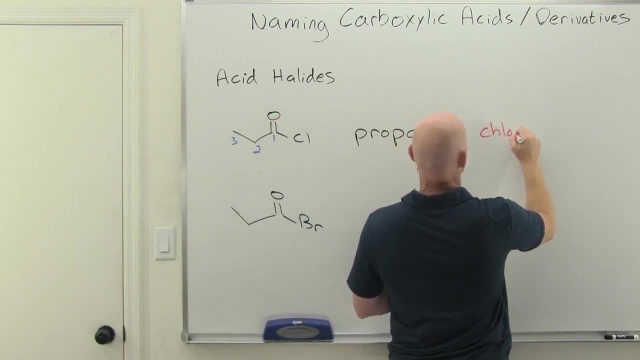 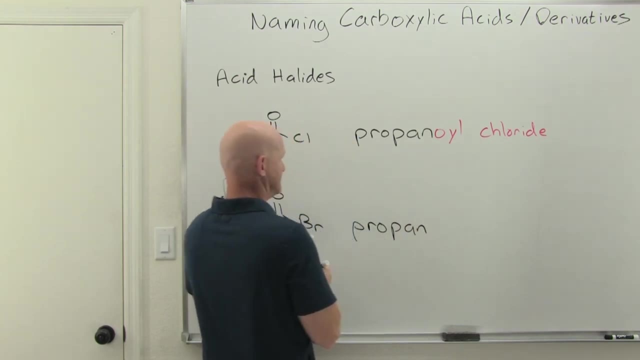 one is this: acid halides is next called acyl halide- same thing. so we'll get an acid acyl chloride and or bromide. So this is propanoyl chloride And the second one here propanoyl bromide. 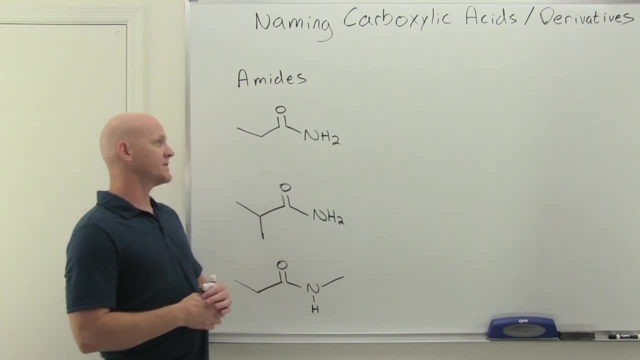 Cool, All right. so we've got amides next on the list. So again carboxylic acids, anhydrides, esters, acid halides and now amides. So here we've got a very simple amide here. 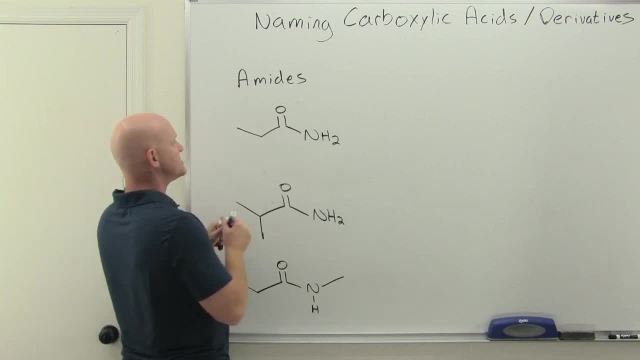 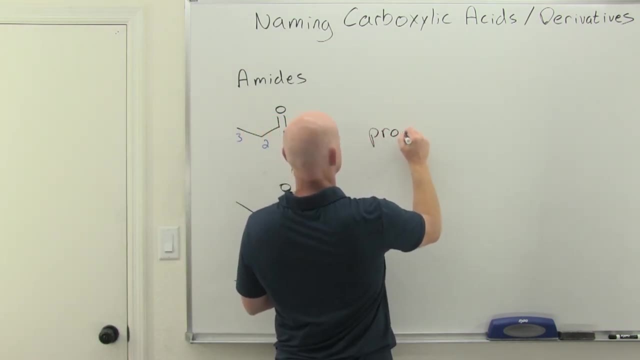 primary amide we say. in this case it's got a three-carbon chain And a suffix for an amide is just amide. So we're going to say propane And because the amide suffix begins again with a vowel sound, we'll drop that e on propane. 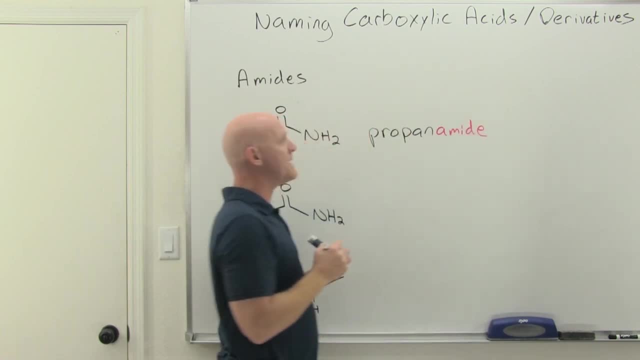 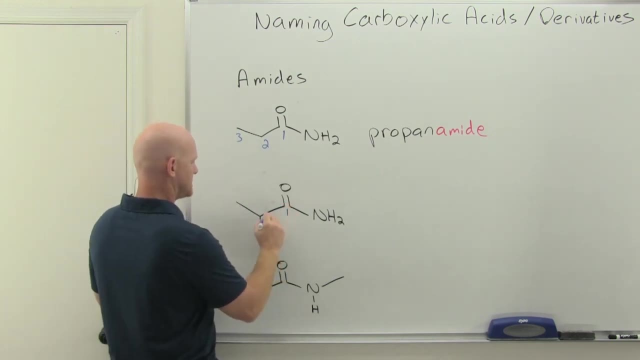 and just say amide, And so this is just propanamide. Now I want you to see the difference here between these next two. So once again we've got a three carbon chains, So one, two, three, and now we've got a methyl group on carbon. 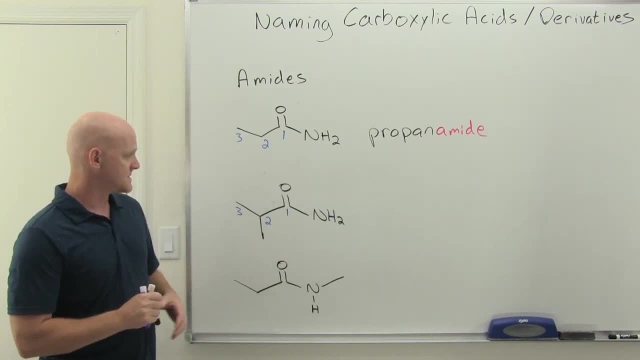 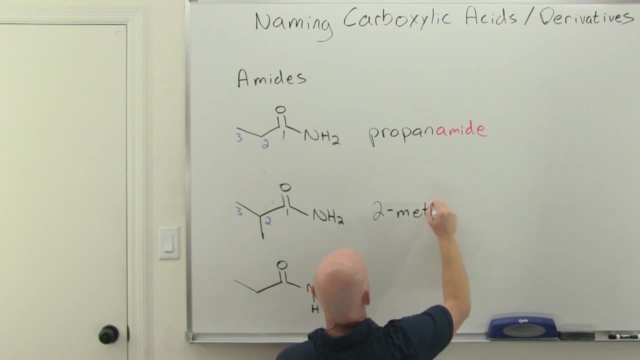 two, And, just like with any other functional group, We'll put those substituents, name them out front. And so here we've got 2-methylpropanamide. Cool, And I didn't really care about this second one, truth be told, but I wanted you to see the. 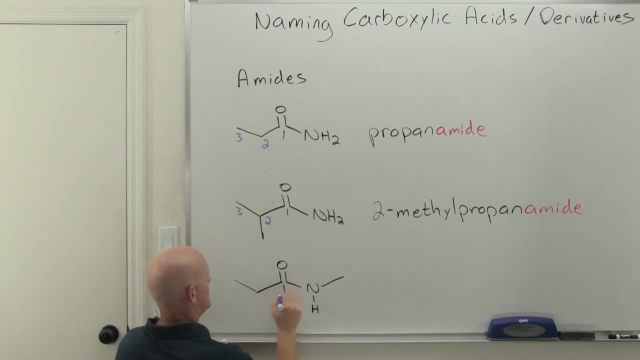 contrast with this last one here. So one, two, three, So we've got a three-carbon chain again, And we've got this extra methyl group right here. So, and this nitrogen even has room for another carbon bond. If we had another alkyl group, we'd call this a secondary amide. So, and what happens? 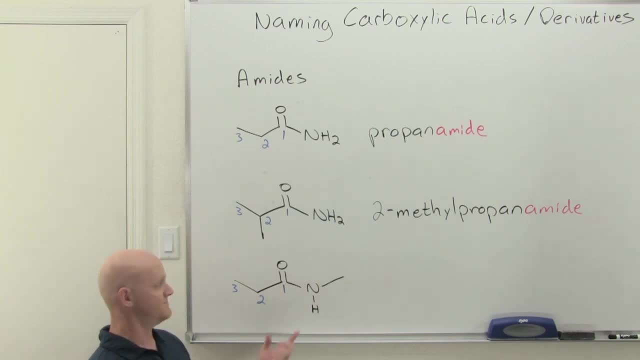 when you've got an alkyl group coming off, your nitrogen here as well. So well, we've got to say that we've got a methyl somewhere, but it's not attached to one of the carbon numbers of the parent chain. It's attached to the nitrogen, And so this is a case where we actually use the. 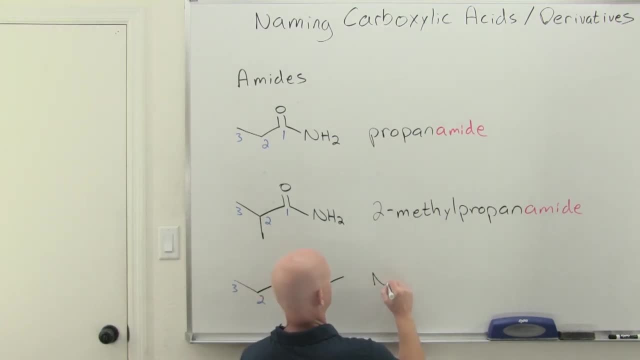 nitrogen as the chain locator, And so this is going to be N-methyl, the capital N, So that actually functions as a chain. Typically, your chain locators are numbers, but here it's going to be a capital N. So and then? 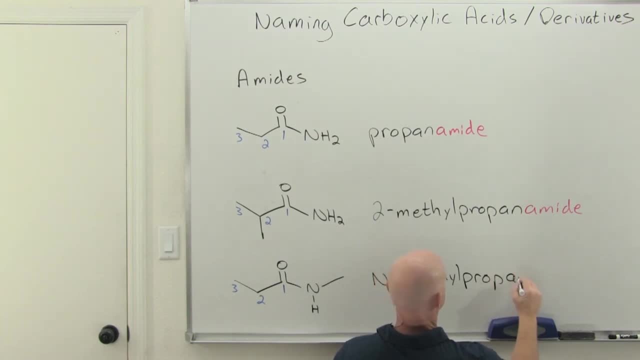 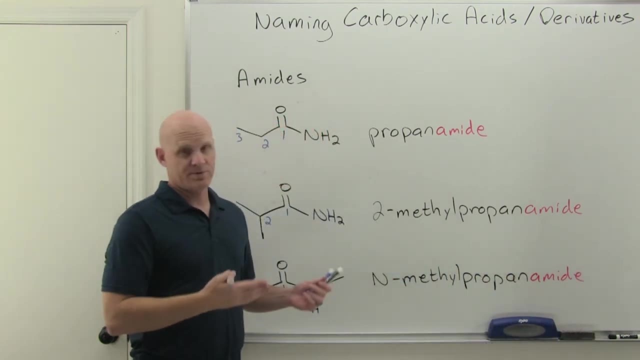 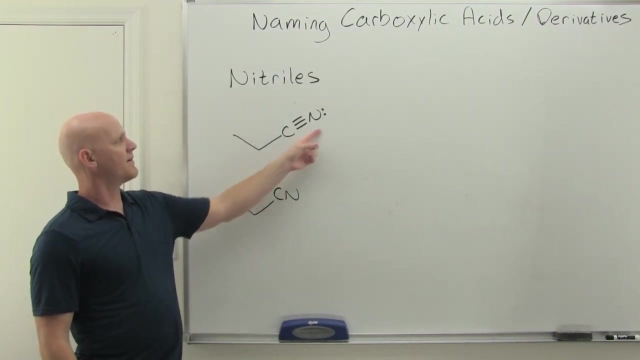 again propanamide. Cool, That's what you need to know about naming amides. All right, So the last carboxylic acid derivative we've got here are the nitriles, So they've got that carbon-nitrogen. 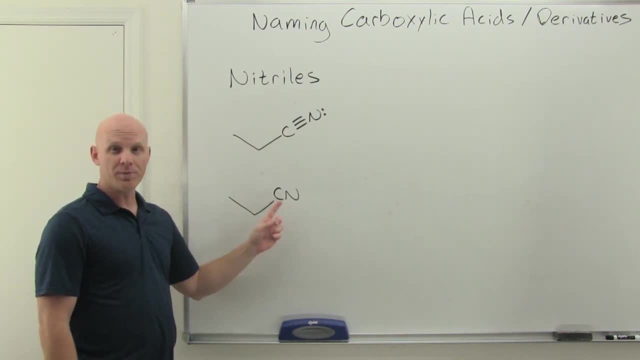 triple bond, the hallmark, And when they're not drawn out, you see that cyano group pretty easily. but these are nitriles And, once again, they're always going to be located at number one. They're always going to be at the end of the chain.